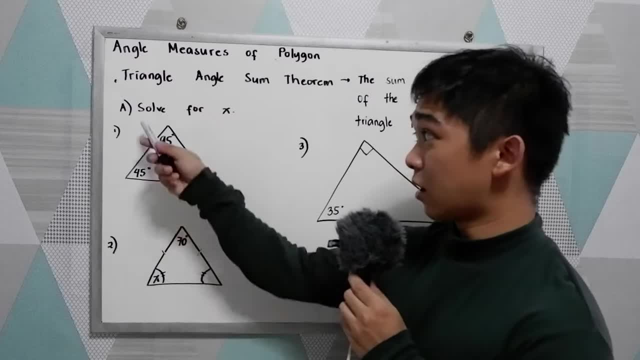 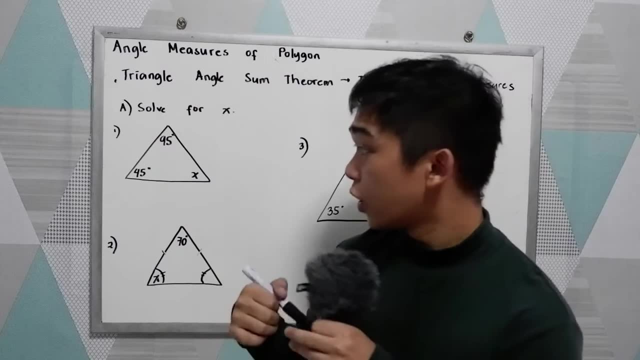 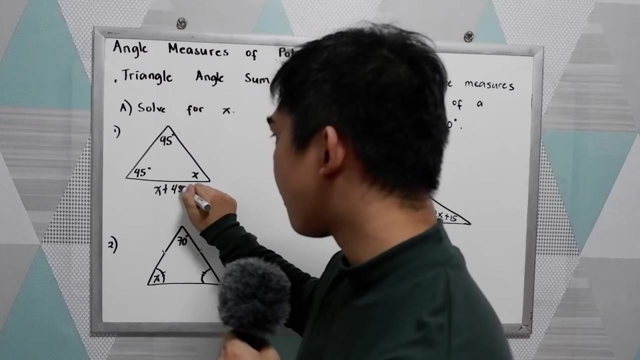 Now let's have our problem number one: Solve for x. So we have 95, 45, then we are going to find x. We know that if we are going to add x plus 45 plus 95, that is equal to 180 degrees. 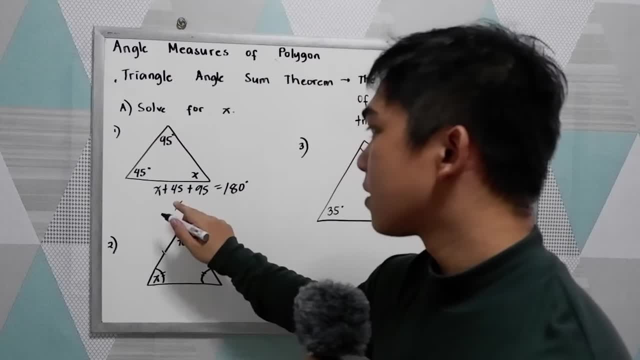 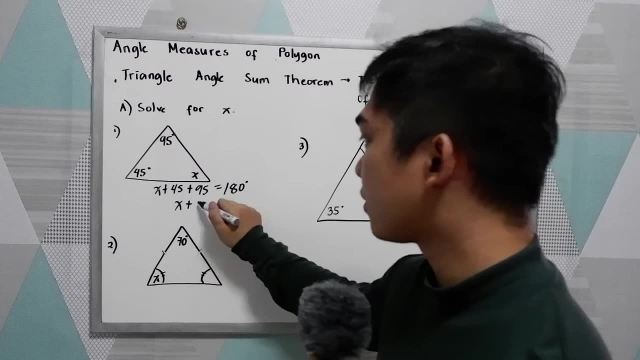 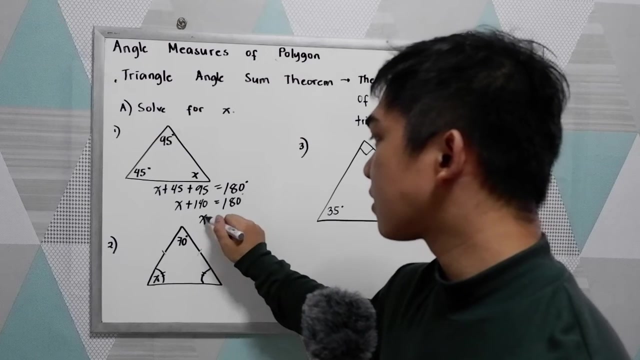 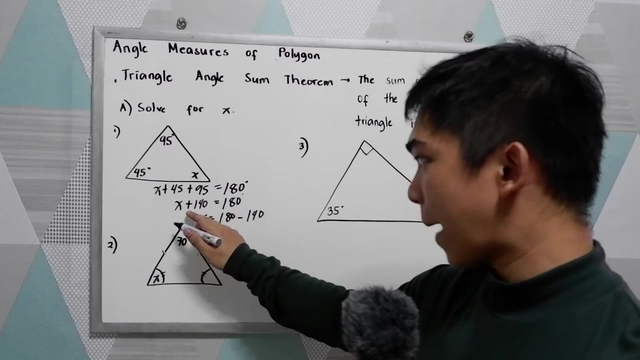 Now x, add 45 and 45. 45 plus 95, that is 140, is equal to 180 degrees. Now we have x is equal to 180 minus 140.. Move the positive 140 to the right side. that will become negative 140.. 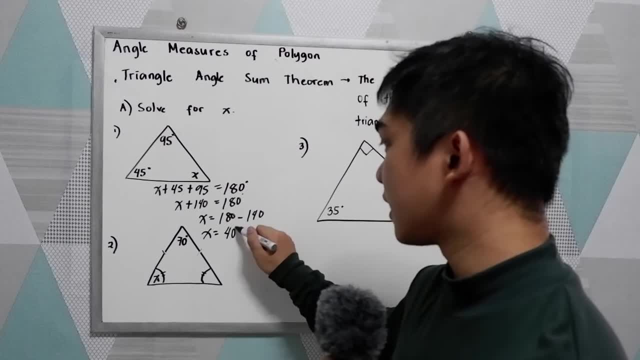 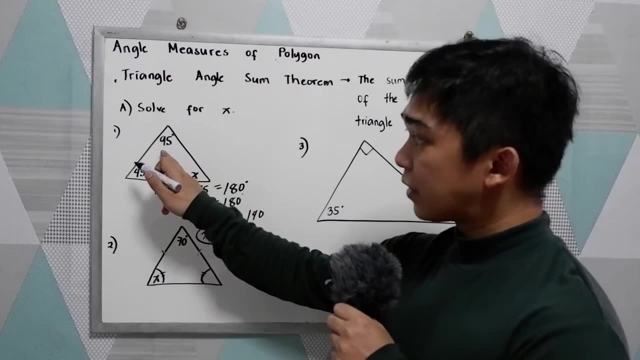 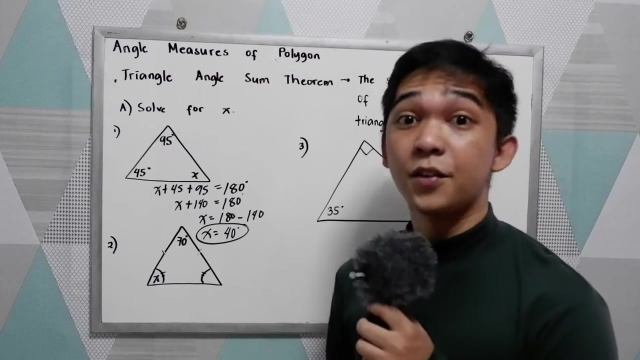 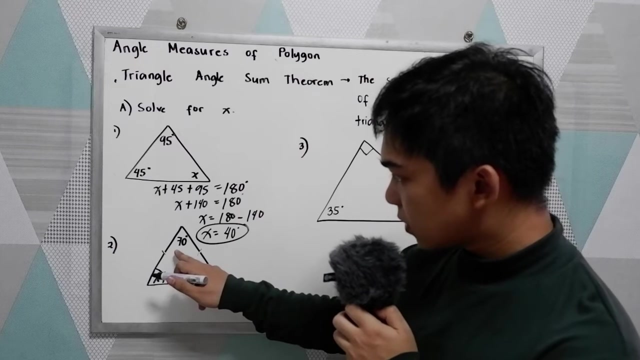 So x is equal to 40 degrees, So our x here is 40.. If you want to check, 95 plus 45, that is 140.. Plus 40,, 180.. Now number two Solve for x. We have the given x, then 70,, then unknown. 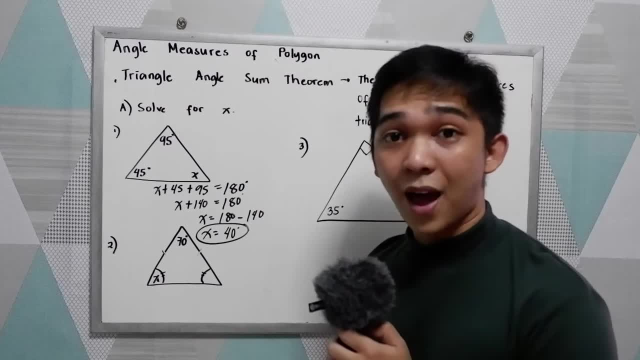 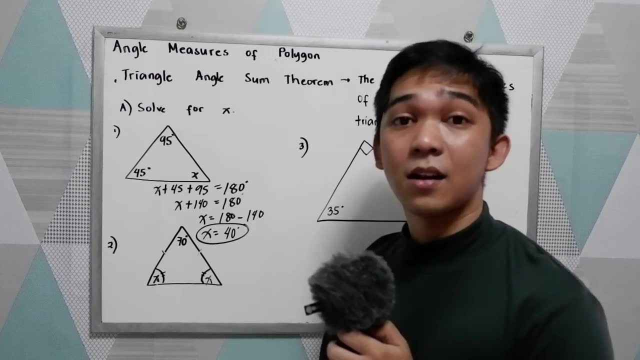 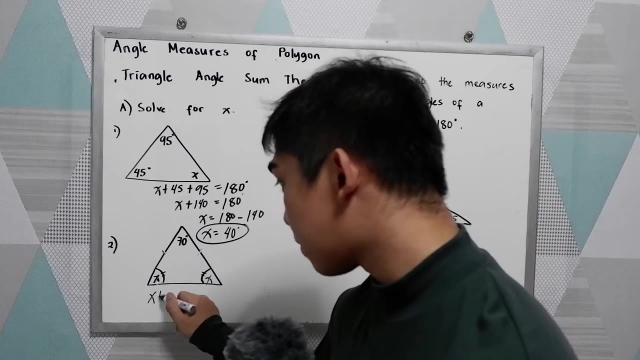 Study our given. So this is an example of isosceles triangle. If this is x, this is also x, because base angle of an isosceles triangle are equal. Now we have x plus x plus 70 is equal to 180. 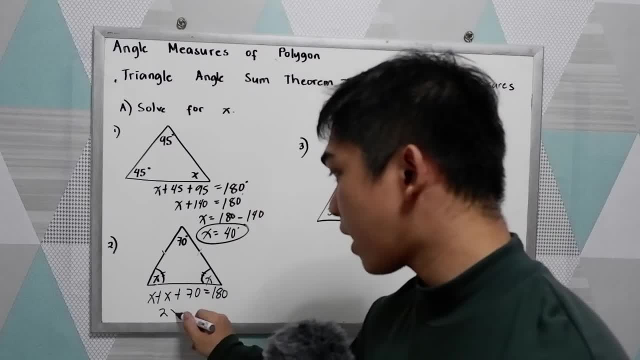 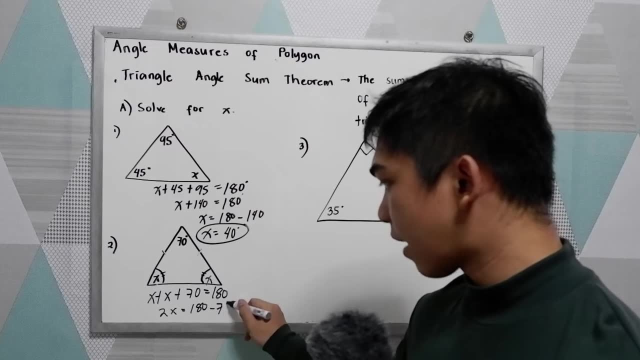 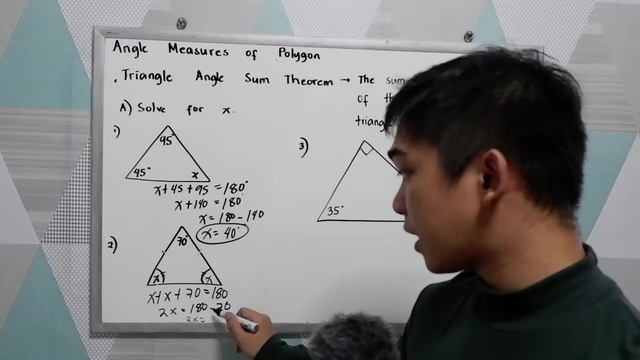 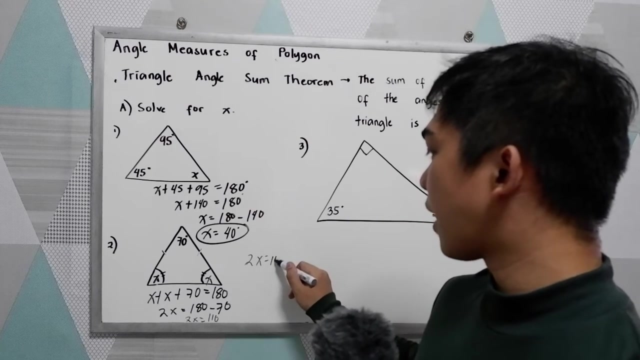 Now we have: 2x is equal to 180.. Move positive 70 to the right, that will become negative 70.. Now we have: 2x is equal to 180 minus 70.. That is 110.. So 2x is equal to 110.. 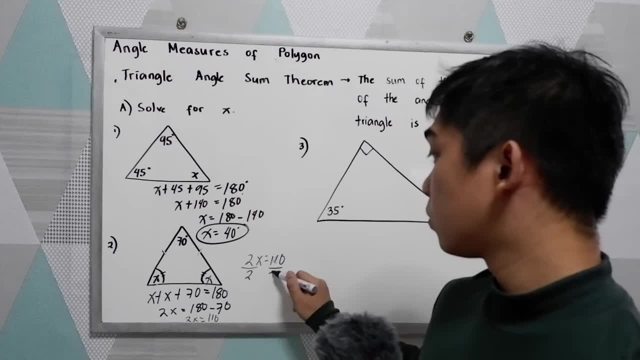 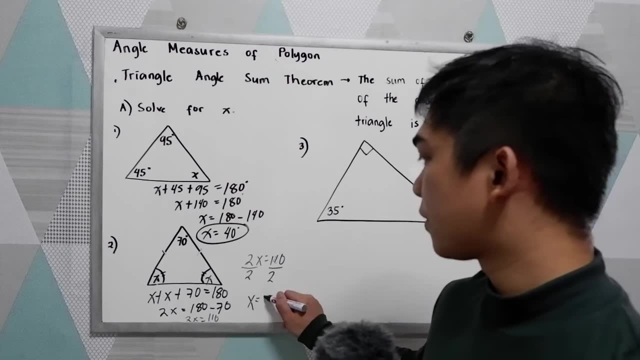 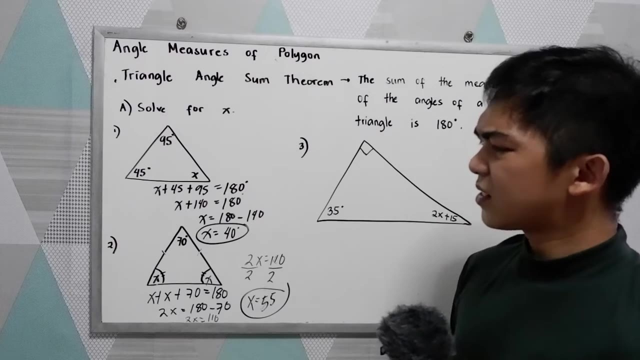 So divide by 2.. x is equal to 110. divided by 2. That is 55.. So x is equal to 55.. So let us check: 55 plus 55,, that is 110.. Plus 70,, 180..